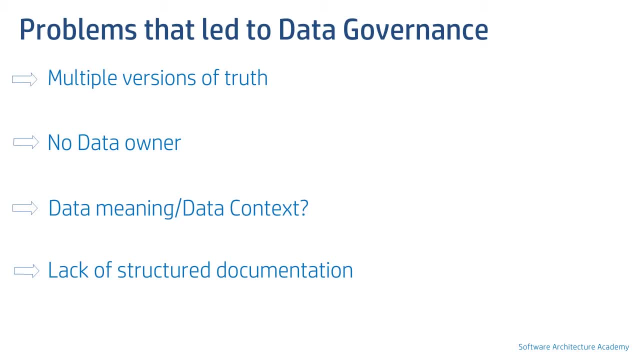 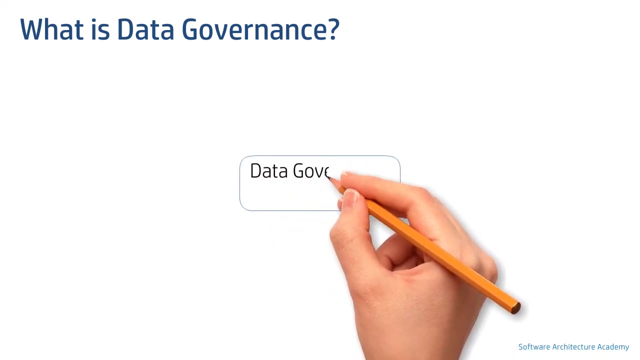 in a standard defined at a enterprise level. This will make sure there is less reliance on people to understand the data In simple terms, data governance is a process of establishing accountability and return of data in all aspects in and around data. this is a field which has seen rapid adoption by large. 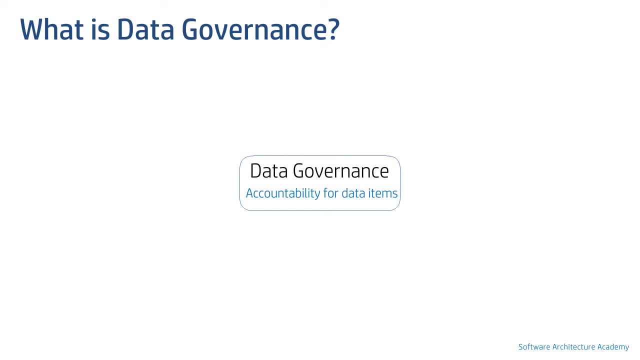 organizations past decade at an unprecedented pace, because organizations have understood the importance of not maintaining a bad data. now we will be discussing various areas within data governance. a lot of these may seem interconnected and overlapping, but that's how it is structured. also, certain organizations choose to categorize master data management, or MDM, under data. 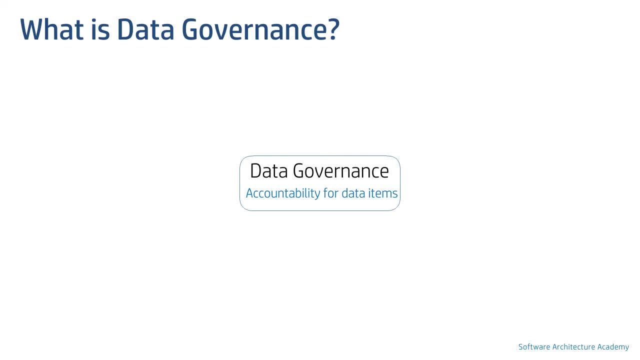 governance, but we will be categorizing it under data warehousing concepts for effective learning experience. so let's get started. data steward ship is the accountability that we just talked about. data stewards are basically data owners. traditionally, ownership have been at an application level, business level or a product level, but data 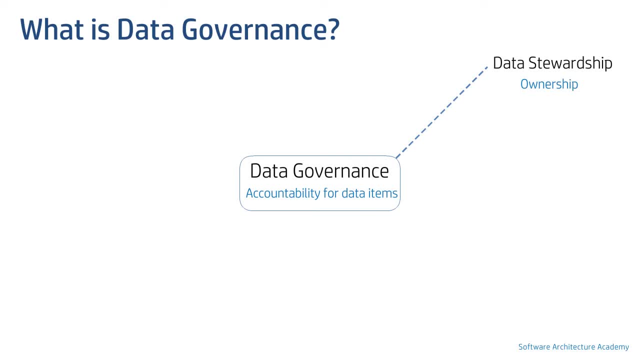 an overarching entity amongst all these aspects. hence it becomes important to establish ownership of data as well as, which leads to the data stewardship program. next, data policy is a set of guidelines to manage things in and around data effect effectively. data policy is usually formulated by a data 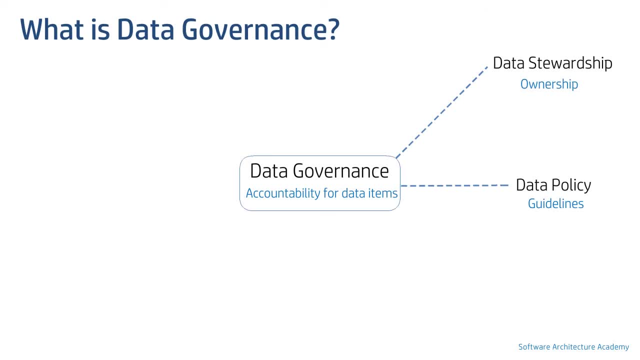 governance council, which consists of data related executives and key personnel's in an organization with adequate representation from all lines of businesses. next, data standards ensure consistent way of capturing, recording and maintaining data across an enterprise. we will partly discuss the example standards and data lineage and metadata management videos in this very series. next, meta data management. to be able to 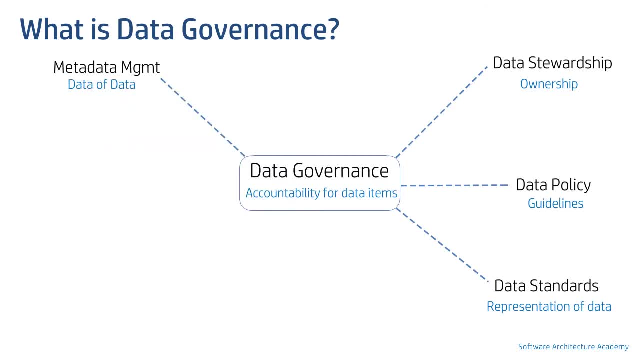 locate a data. we use metadata, metadata management, decent capturing, recording and maintaining metadata. This will be covered in a separate video. Next, data lineage is tracking data movement to its origin, along with recording transformations. We have a dedicated video on how data lineage is captured and it is explained via illustrations. 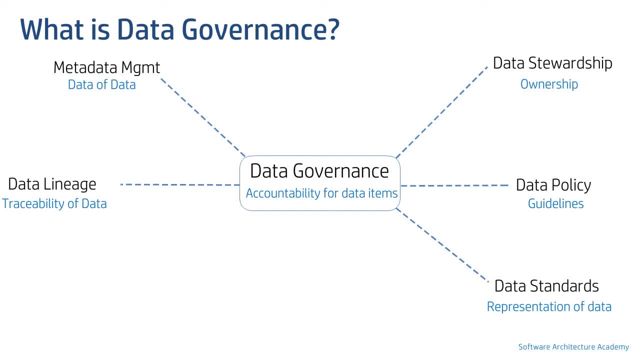 It also talks about the ways to build a lineage system. Do check it out. Next, Data Cataloging involves business glossary creation and, most importantly, it links technical metadata and business metadata. What is technical and business metadata? Do check out my other video on metadata management. 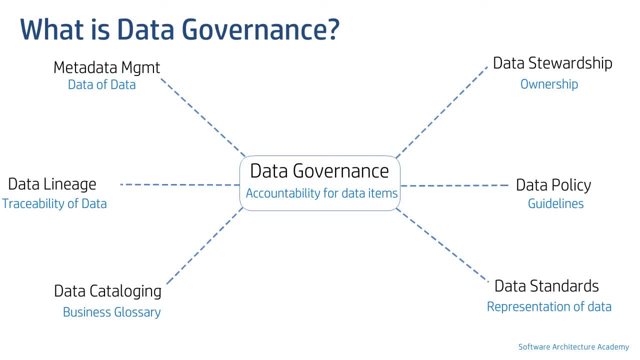 It explains in details, along with real-world examples. Data cataloging will also be covered in that very same video. Next, Data quality is basically measure of data's usability and is very important to ensure data can be stored. So Bet them out. 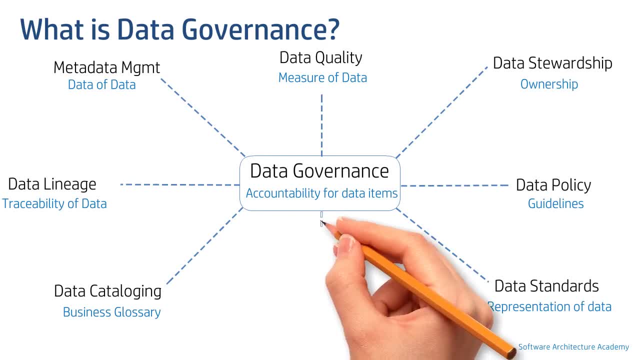 serve its purpose. This will also be covered in separate video. And finally, data security deals with security related aspects like access management. One key aspect that data security deals with these days is detecting and flagging PII, which is personally identifiable information. 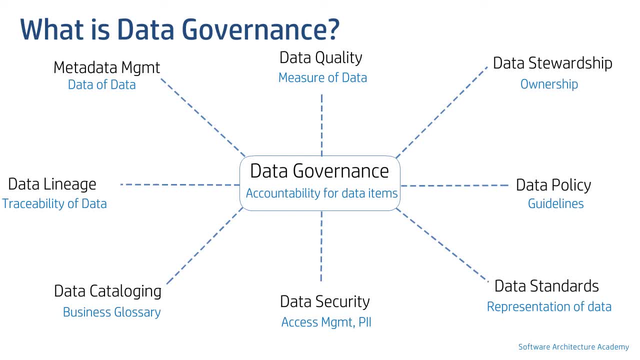 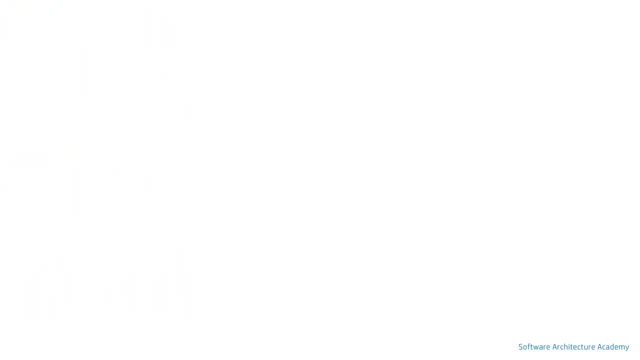 This is critical to regulatory compliance like GDPR. So what is trending in the world of data governance? Various vendors like Colibra Informatica, ASG, IBM, etc. have a wide range of data governance products in the market. They are working very actively to expand the capabilities using latest technologies. 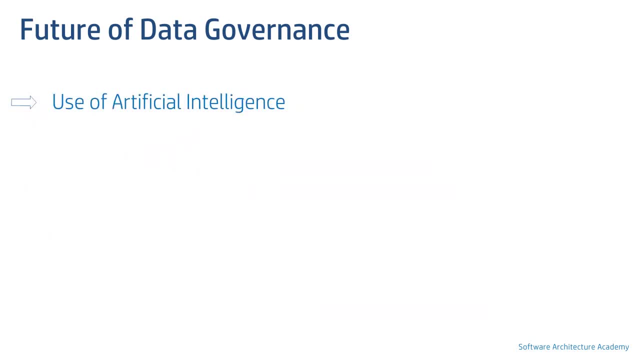 First, use of artificial intelligence in data governance is evolving. Key areas are data cataloging using NLP, which is natural language processing, linking technical and business metadata using machine learning and natural language processing. and data quality checks using AI. Consider all the challenges that we discussed at the start of the video. If data is defined. 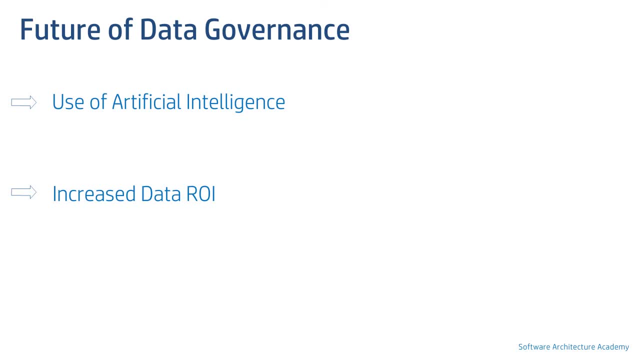 ownership established and there will be a single source of truth, return on investment on data-related initiatives can increase. This has already started to reflect in large organizations. So that's all we have for today, If you liked this video and had a good learning experience.